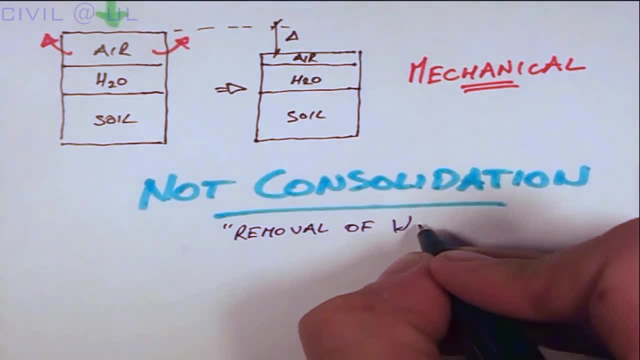 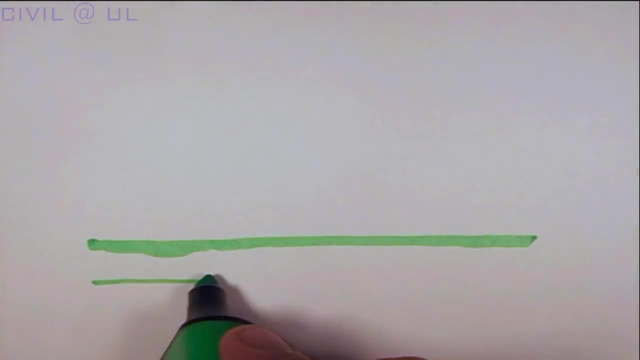 which is the increase in soil density as a result of expulsion of moisture. As we saw earlier, this is a time-dependent process controlled by the permeability of the soil. There are many techniques for compacting soil. Here are some of the more common methods For coarse-grained soil: 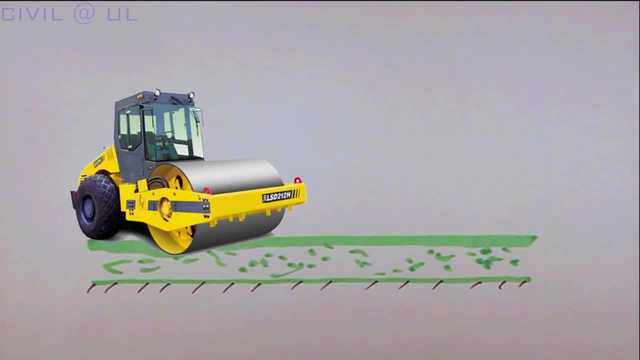 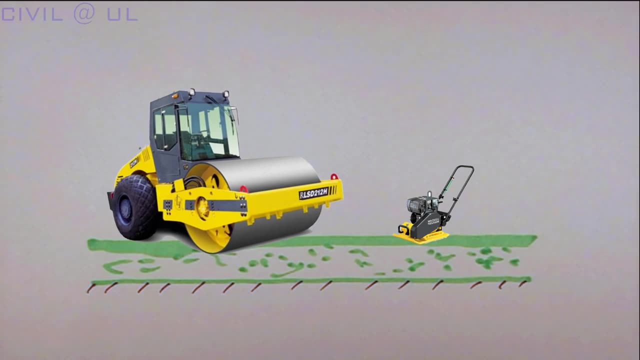 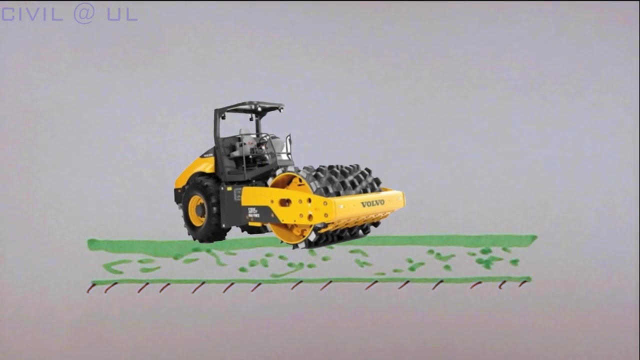 such as sands and gravels. smooth drum rollers are popular And, for small areas, whacker plates may be used. For fine-grained soils such as clays, sheep's foot rollers or pneumatic rollers are more popular. This equipment is typically effective for relatively shallow lifts of soil in the order of 250mm loose. 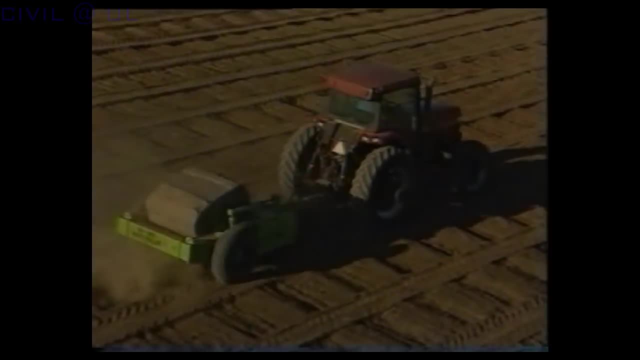 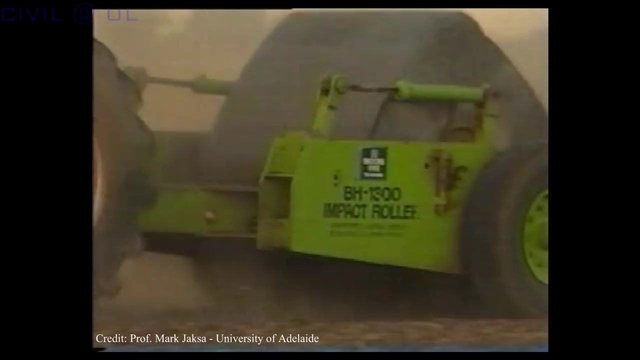 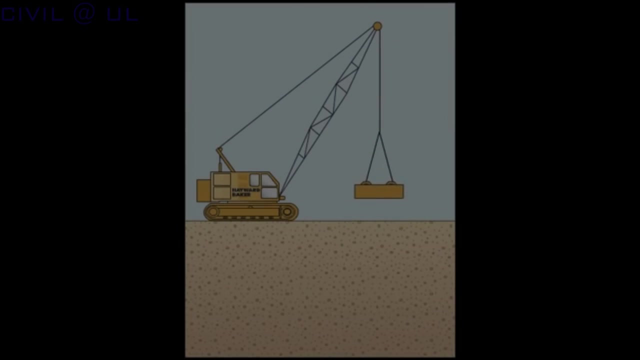 lifts. For deeper compaction of coarse-grained soils, an impact roller may be used. These are effective up to depths of approximately 1m and have a much higher operating velocity than the smooth drum roller, so they are much more efficient. Even greater depths of compaction can. 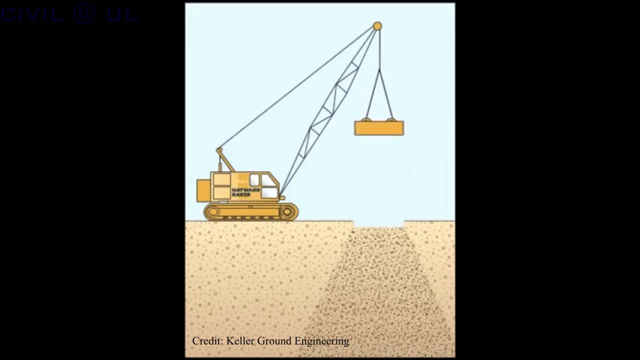 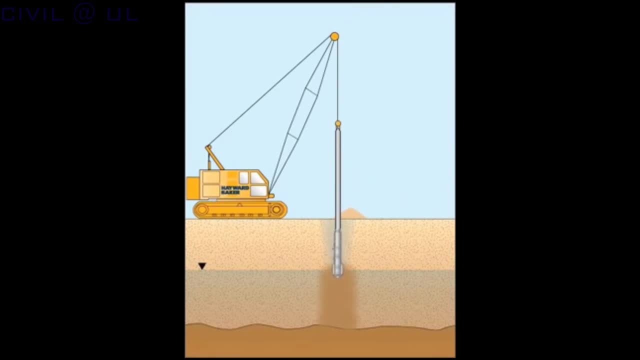 be achieved by using dynamic compaction or fibro-filtration techniques, Although these methods have limitations when operating close to existing structures. I encourage you to read the literature and search the internet to learn more about these methods. If you have any questions, feel free to. 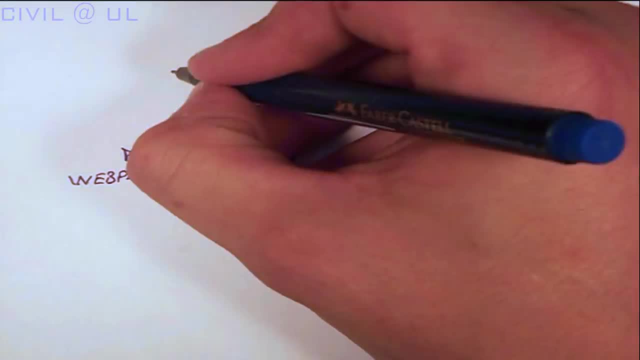 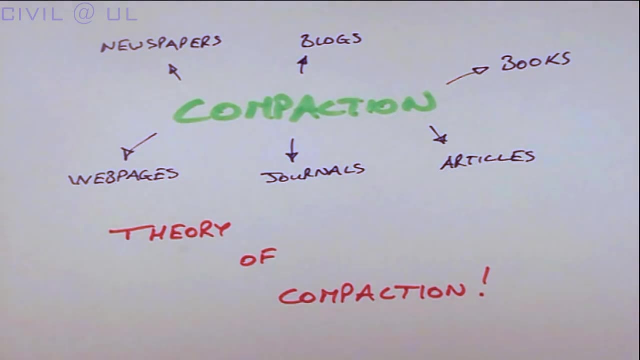 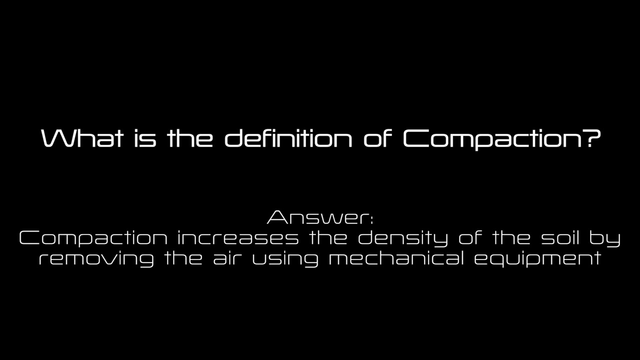 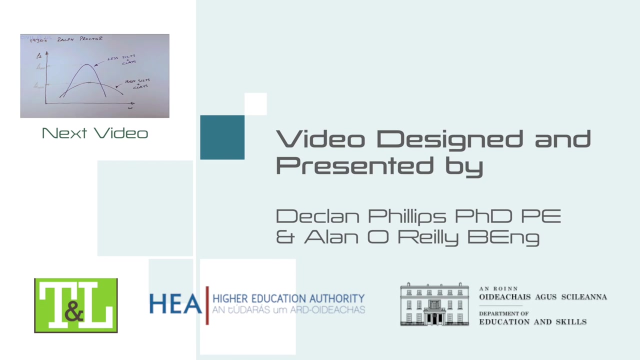 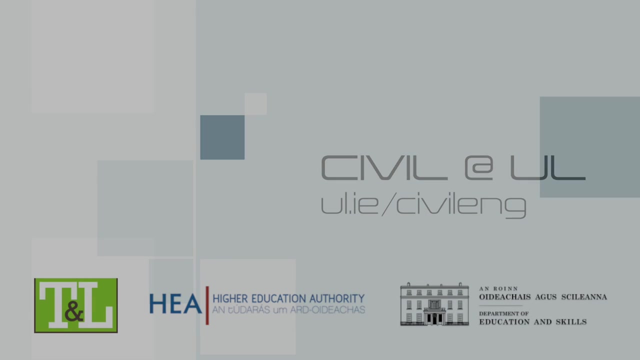 contact me on the internet for additional information and videos on the compaction process. We will now turn our attention towards the theory of compaction, But first a quick quiz question: What is compaction? What is compaction?